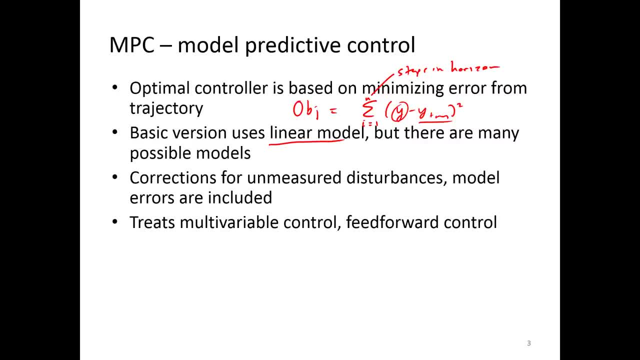 Now, the beginning applications of MPC had linear models, But there's many different types of models So these can be linear, empirical. They can be first principles. I know those are generally nonlinear. OK, combination of the two and those would be something like hybrid, hybrid models. 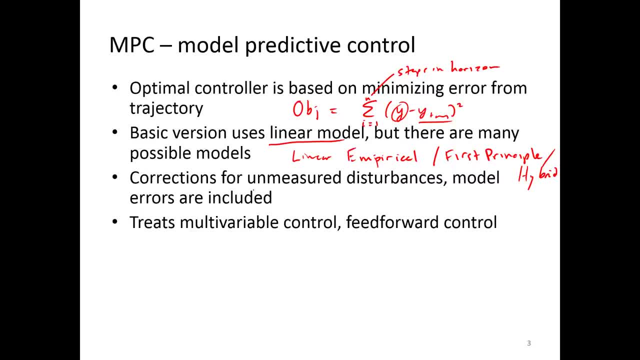 okay. what we want to do with these, these controllers, is to reject unmeasured disturbances, things that affect the process and drive it away from that target, and also be able to treat multivariable control, also be able to include maybe some information about feed forward. let's say it's going to be. 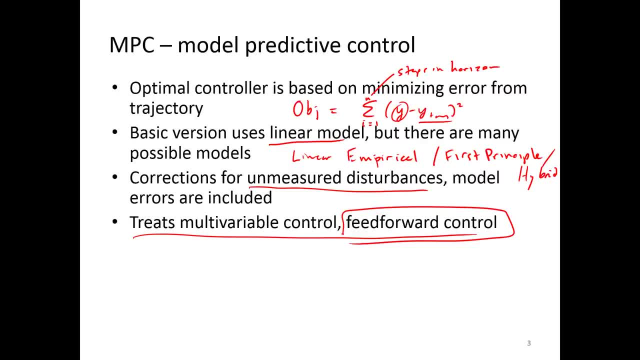 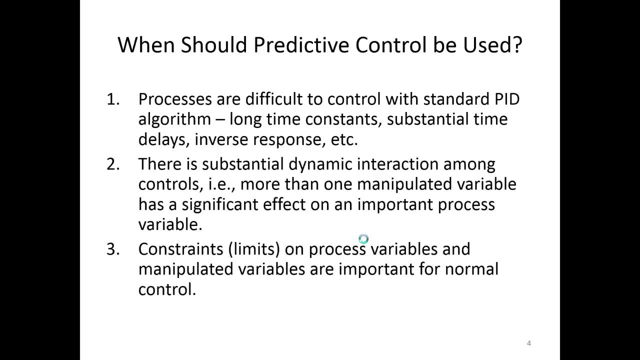 raining. we might be able to take that information into account in a distillation column and proactively correct for it. okay, so why should model predictive control be used versus, you know, standard PID controller? a couple cases where where it really benefits are in long. you know processes with long. 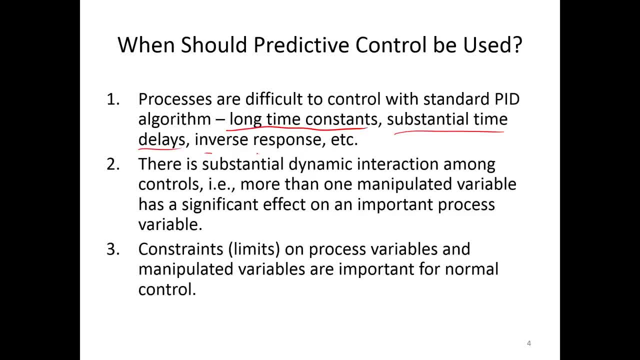 time constants. you know delays, inverse response, that's just for for single input, single output. also, you know, if you have multiple manipulated variables and control variables that all affect one another and model predictive controller can take those into account, whereas no PID controller, you may have to have some sort of feed forward mechanism and 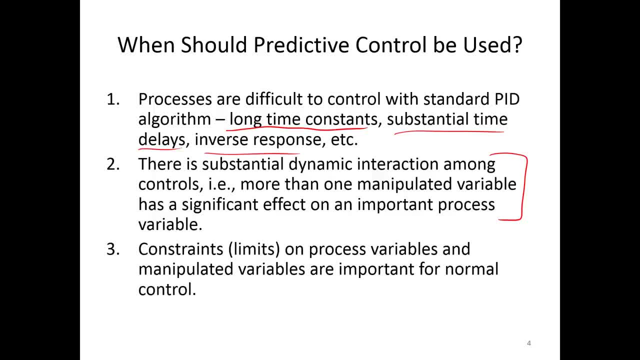 information sharing between the controllers. so model predictive controller that does that, naturally you're able to get some of those interactions, exploit that information in the controller. also, you know if you have constraints on the limits. you know, either for manipulated variables, let's say a valve that can only go between 0 and 100% open, or a pump. you know the. 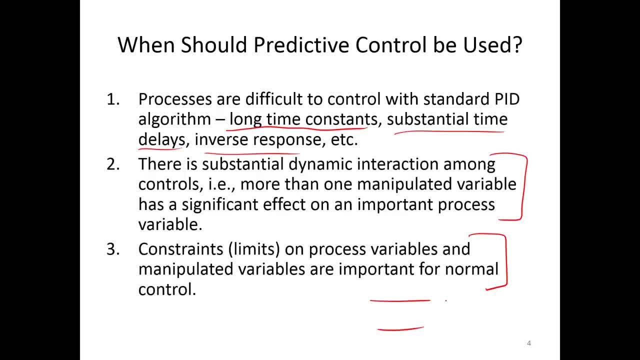 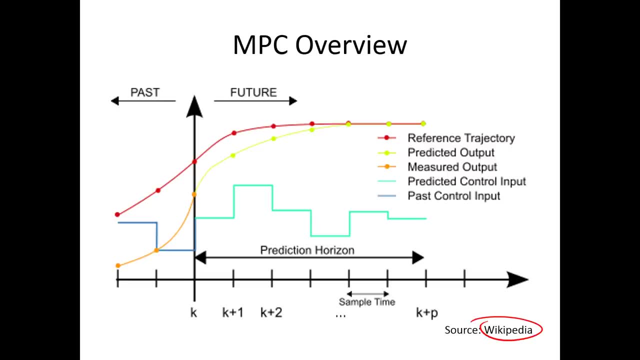 flow rate or also for constraints. you may have upper and lower limits on that and want that variable to stay within those limits instead of necessarily driving to a target. okay, so here's an MPC overview. it's just a simple schematic taken from Wikipedia. you have your manipulated variables and typically you 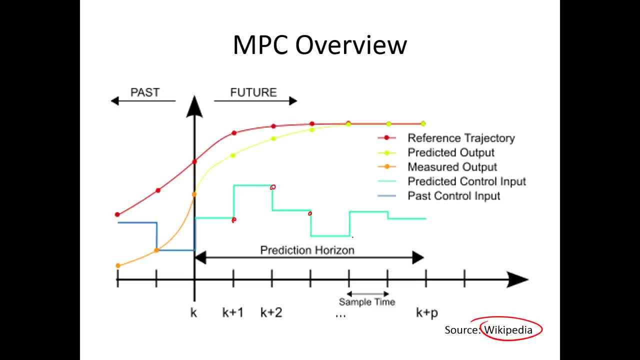 you make discrete decision points into the future, you know where that manipulated variable is going to be, and and then you also have process. okay, so these are your measurements right here. okay, those were, those were your measurements that came from your process variable that you're trying to drive to a target. so let's say, this is for. 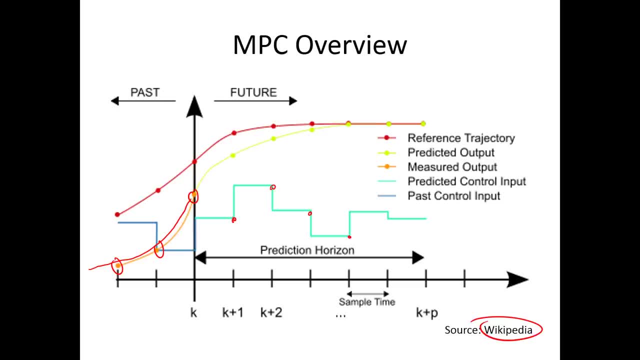 example, a temperature. okay, so you want it to follow this temperature profile and getting up to a target value for that that temperature, and this might be a low rate on a cooling. you know, on a jet on a jacket, react on a jacket of a, a reactor, and so you're adjusting this in. 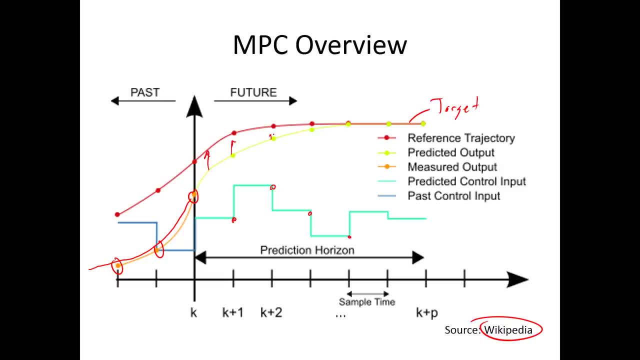 order to be able to drive this closer to the target and, and considering all of these points into the future, okay, to try to align that and that's where our sum of squared errors came from. you know Y minus Y trajectory and you might have a squared error. okay, so you're going to be. these are going to be a degrees of freedom. 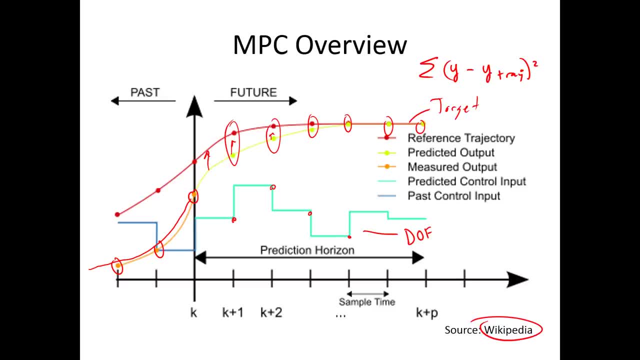 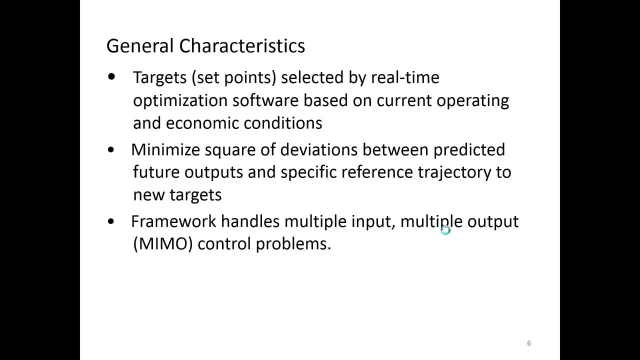 that you can adjust or that the optimizer can adjust in order to be able to drive you to your target. Okay, so we have targets that may be coming. you know, those may be changing as well. That might be coming from another application that's optimizing maybe the whole. 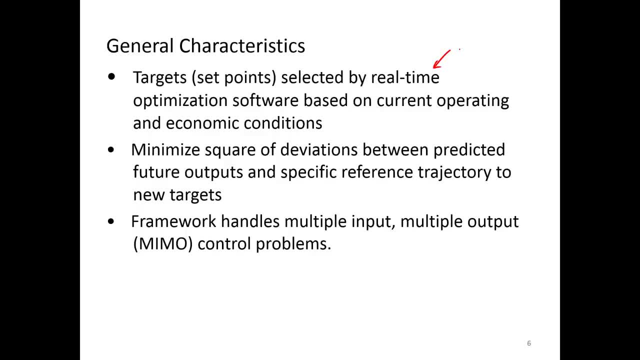 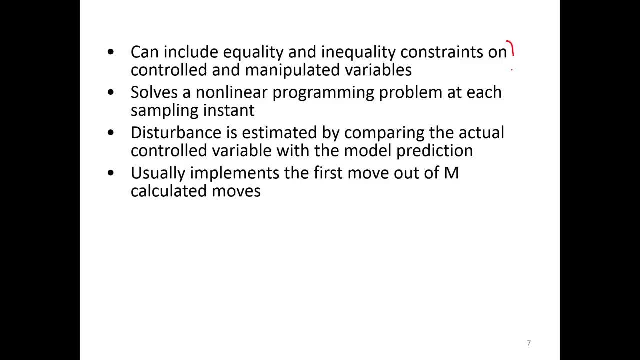 plant or the, you know coordinating between multiple controllers. And you know with, the important thing with model predictive control is it can handle multiple inputs and multiple outputs or MIMO control problems. Okay, and then we could also include equality and inequality constraints on the controlled and manipulated variables. So it's a constrained. 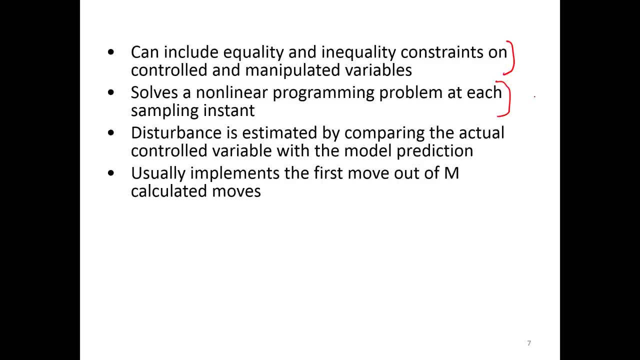 optimization environment. You know many packages have the ability to solve linear or nonlinear programming problems at each sampling instance, And then we're also able to estimate disturbances. If we can do that better, that's kind of like a feed forward we're able to take. 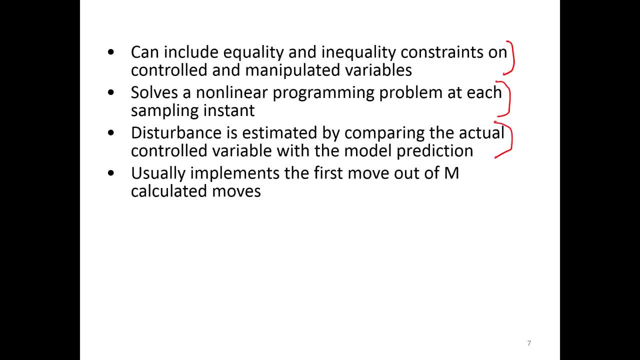 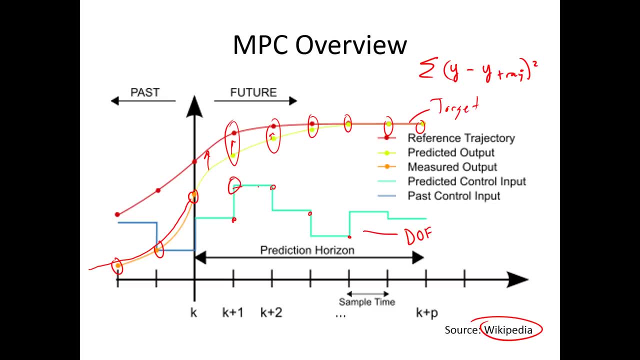 that into account. Okay, and then the important thing with MPC is that we're just taking the first move out of the total calculated moves. So what we're doing is just taking this move right here, and that will actually be implemented in the process. Now the next time step. 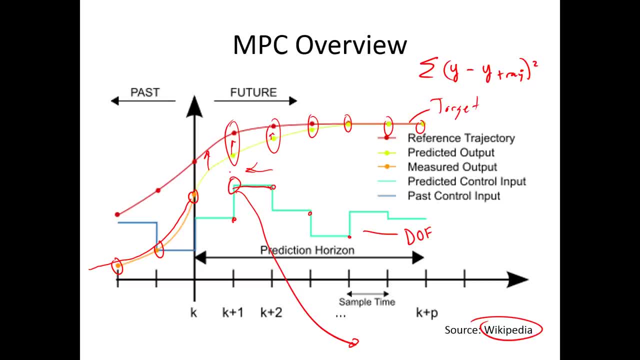 everything shifts over by one. and then you recalculate your moves based on this new measurement that might arrive at this time point, And then you would implement this move, Okay, and that would be implemented. everything else thrown away. and then it would cycle again at the next sampling period, Okay, so now we have just a single. 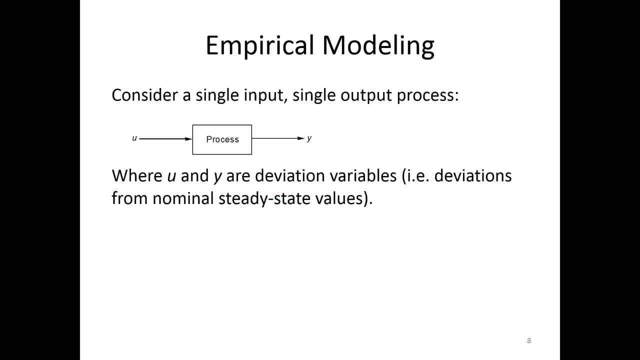 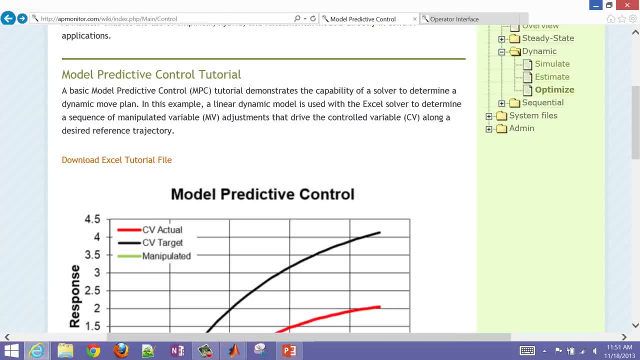 input single output process. What I'm going to do is switch over now to a. let me go ahead and switch over to a website where we have some of this information, If you just come to the apmonitorcom website. here is the address. 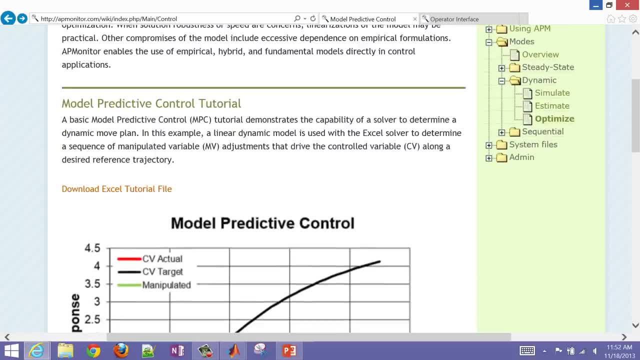 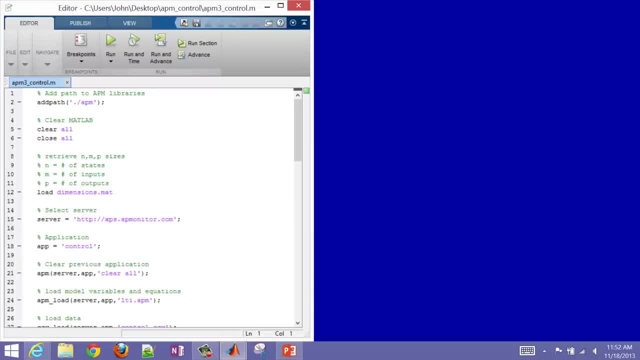 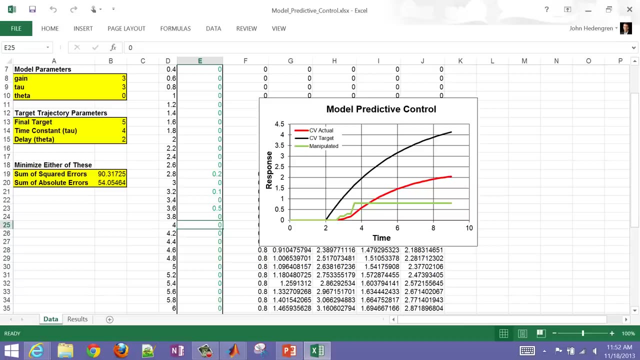 Okay, so I'm going to go ahead and go ahead and download this Excel file right here. You know, just doing these calculations in Excel. So what I'm going to do is, once I download that and extract it, open up the Excel file and what? 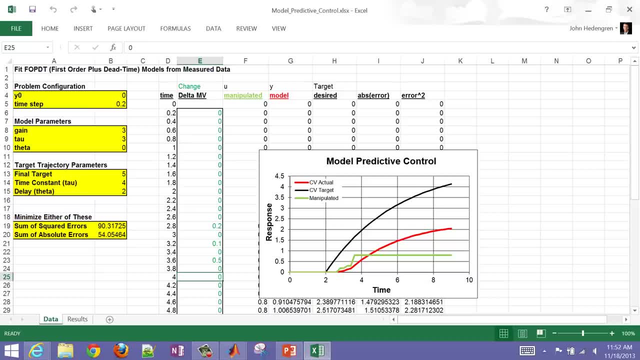 you'll see is just a very simple interface here that shows a manipulated variable, a model and then also a desired target. So this is our desired target. Okay, the black line here is our desired target. So this is our desired target. 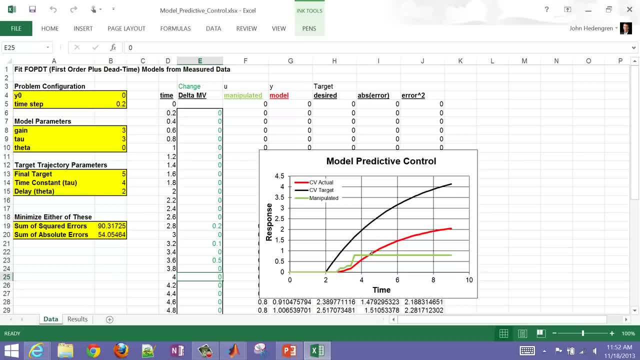 The black line. that's where we want to drive our process response And we also have a red line here and that's that's going to be the process model. So if we, if we have this sequence of moves given by the green, that's going to be our 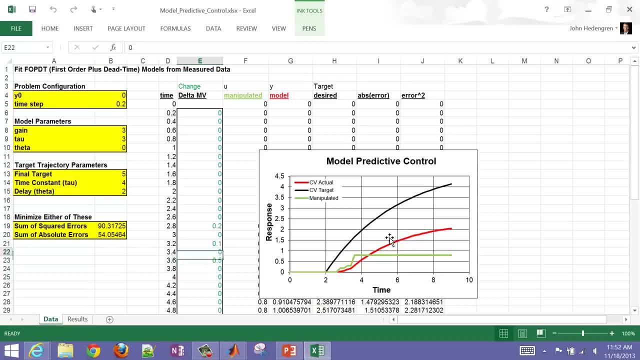 response: Okay. so what I'm going to do now is go ahead and just change that. Okay. so I'm going to add this is: these are the delta moves at every time, point. Okay. so I just added one to my delta right at a time of three, And then you 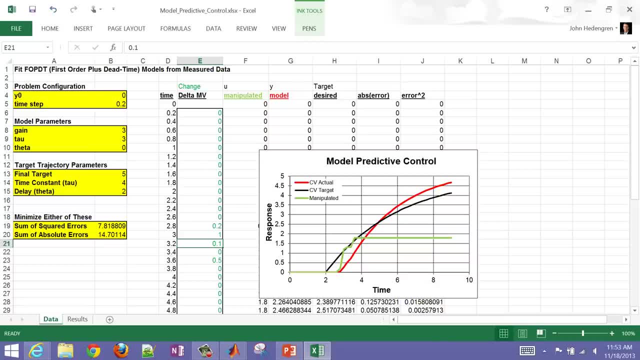 could see how my process is going to change. I'm going to go ahead and set that to one every time. That's the way I'm going to make sure that this actual target changed. Okay, so what I can do is, you know, kind of do this manually if I wanted to. Let's say, I say, well, it needs to go just a little bit faster right here. 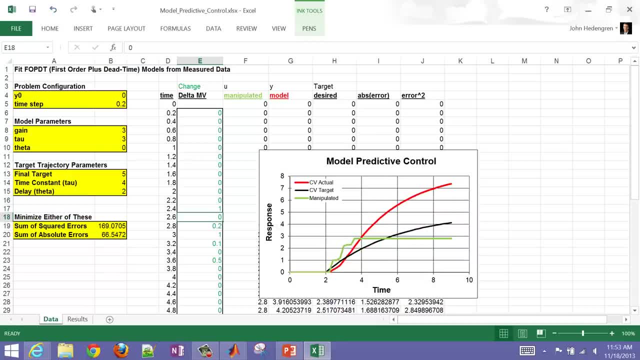 Let me go ahead and enter one in here And it shifts that up. I said, well, I might have gone too far with that move of three down here. Let me take that away. Okay, so it's going to adjust that. you know the actual model prediction, Okay and and be able tovel that. to set up. Okay, so it's going to adjust that you know the actual model prediction, Okay, and and be able tovel that to a small amount of time- Okay, so it's going to adjust that to a small amount of time. 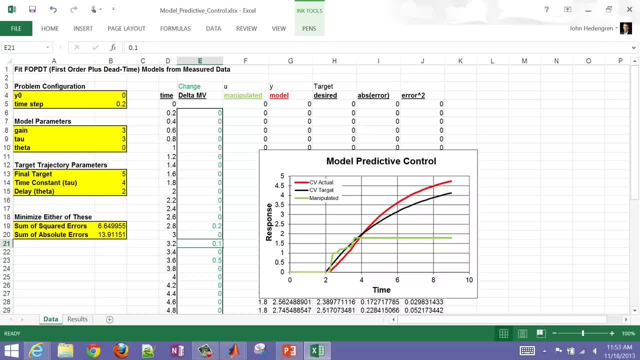 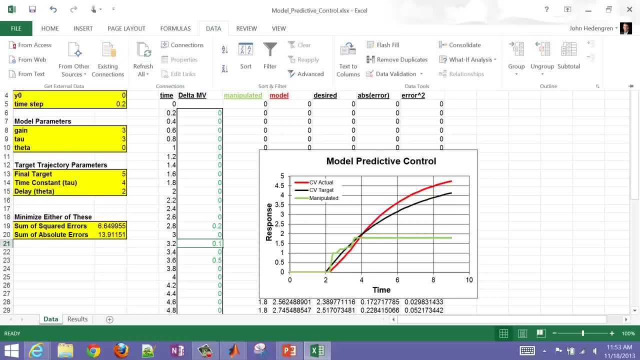 be able to use these degrees of freedom that are shown by the green line, and the solver will typically do this. it's typically not done manually, okay, so one of the other things that we can do is use a solver to be able to solve this, and so let me, let's see if I've got the solver. 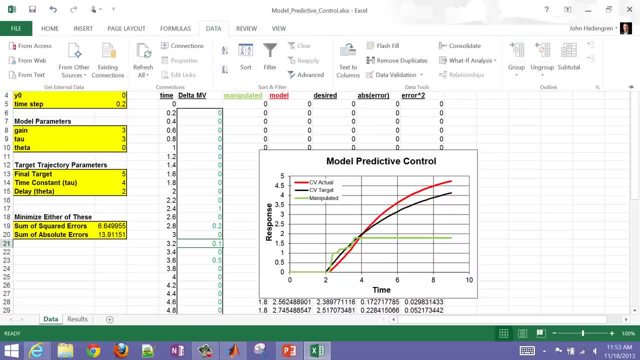 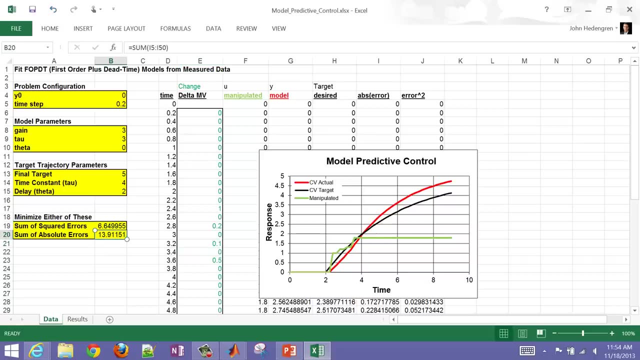 on here. I don't think I have this one installed. let me. let me just check and see if, okay, looks like no solver right here, but but if you have Excel solver, one of the things that you can do is is go ahead and minimize the sum of squared errors or the sum of absolute errors by adjusting. 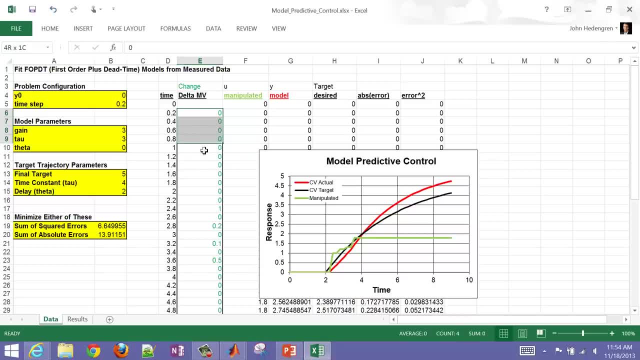 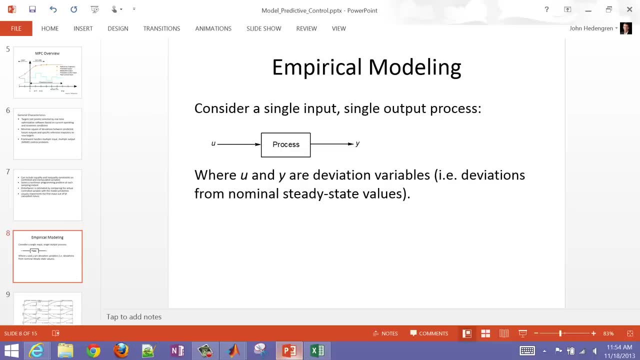 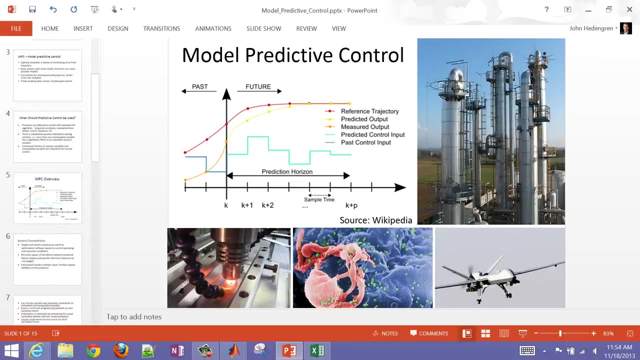 and then adjusting these manipulated variable moves right here to be able to get those to a line, okay, so, so I'm going to go ahead and just minimize Excel, okay, and. And then let me go back to the PowerPoint. Okay, and I'm going to go pick up where we left off here. 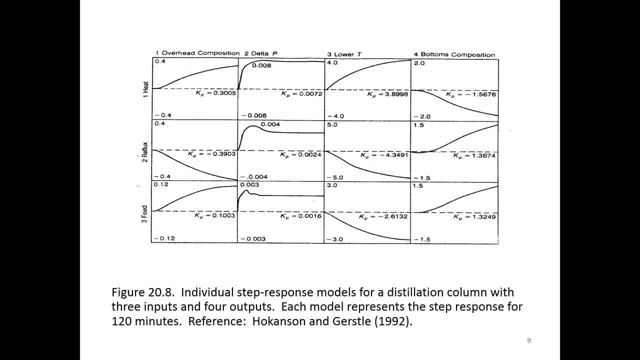 One of the other things that we can do with multiple predictive control. that Excel example was just a single input, single output system, But one of the advantages of multiple predictive control is that you can consider a multiple input, multiple output systems. Okay. so, for example, this might be the heat that we apply in a distillation column. 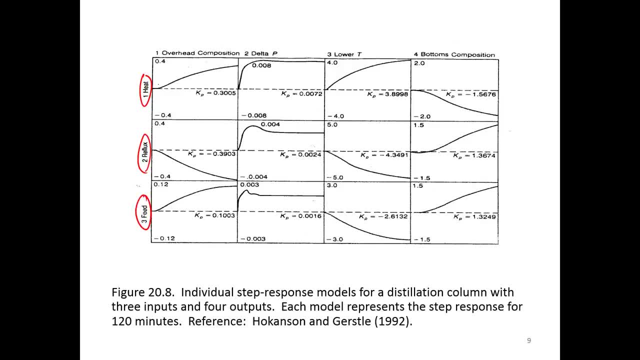 We might have a reflux ratio and then a feed, And then these are our outputs. Okay, so these are the controlled variables. Okay, these are the controlled variables, the things that I'm trying to drive to a target, And then these are: 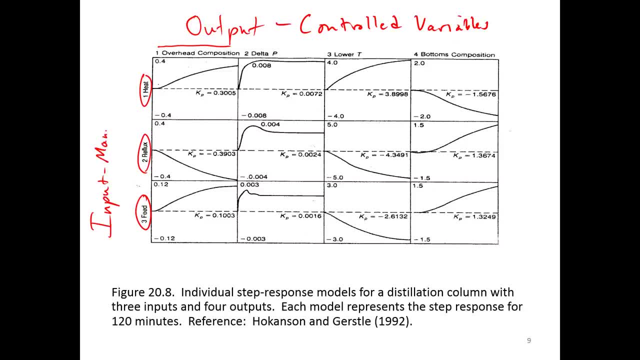 These are the inputs. okay. the manipulated variables: Okay. so manipulated variables on this side, controlled variables on this side. So if I do a step in my heat, the overhead composition is going to increase, The delta P is going to increase. 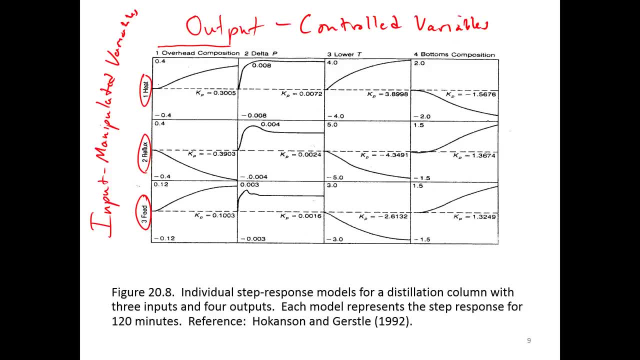 Lower temperature is going to increase And the bottom's composition is going to decrease. Okay, so reflux ratio as well. If I take a step, If I take a step up in that you can see a reflux, The overhead composition goes down. 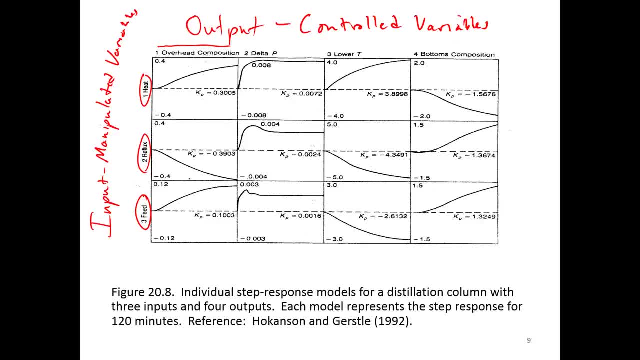 And then you can see these other responses. Okay, so here I have three inputs and four outputs. Now I want to be able to use that model, let's say, to be able to control this distillation column. Example: if I have a PID controller, I might have to pair, for example. 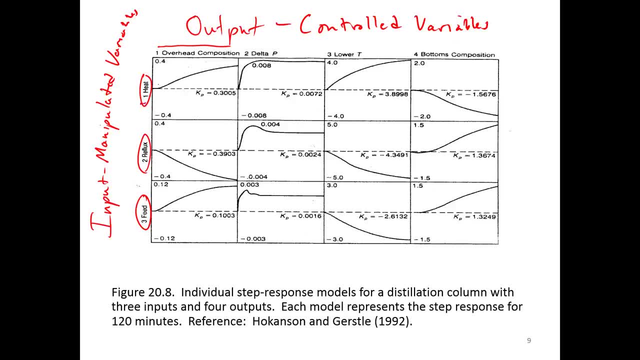 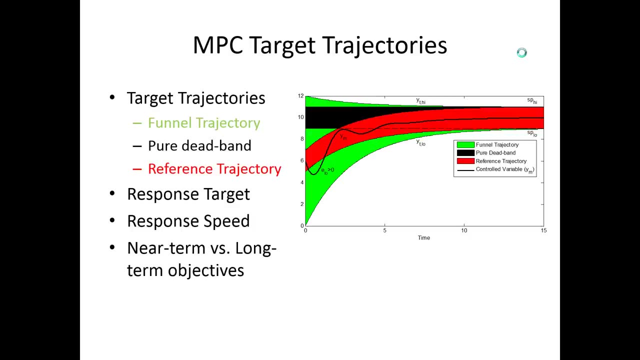 one manipulated variable with one controlled variable. But in MPC you can have different numbers. You can have a higher number of MVs than CVs and still be able to control that system. Okay, the other thing that I'll mention with this is that you may have different trajectories. 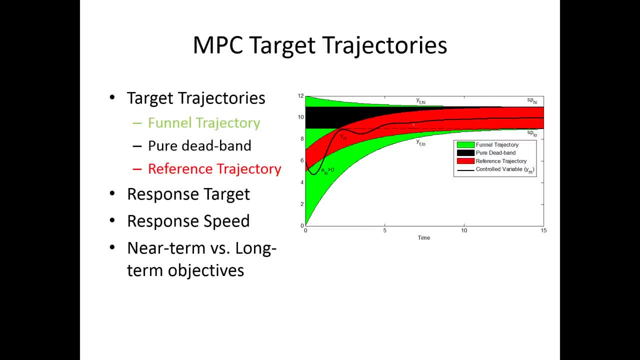 Now we showed in that previous one that just a single trajectory and we are trying to, for example, you know, make it up to this new set point, In this case right here. let me go ahead and change the color here of the ink. 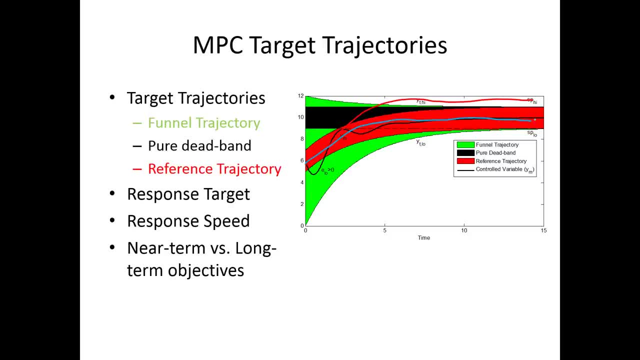 You know. so this might have been the trajectory that we wanted to follow. You can also have a dead band here. Okay, so that's just a pure dead band. You say, well, I wanted to get it up to this dead band as fast as possible. 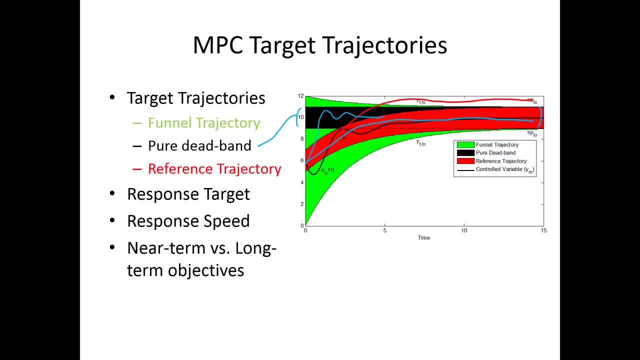 Okay, and then stay within that dead band. You may also have somewhat of a funnel here. okay, as it comes up. So you say I really don't care where it goes in the near term, as long as it comes to a final steady state range. 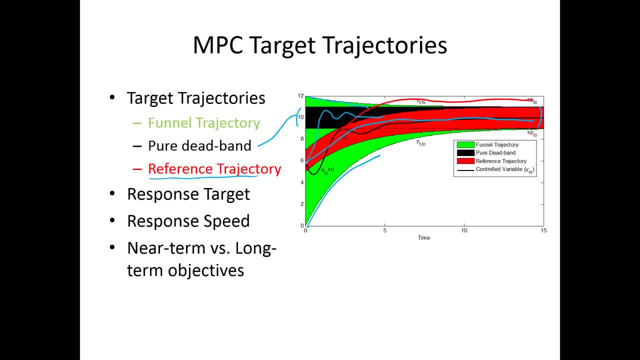 Okay, and then also another popular one are reference trajectories. So here's somewhat of a dead band here, and you know, as long as I stay within that red dead band or the reference trajectory, then I say, oh, I'm doing a good job. 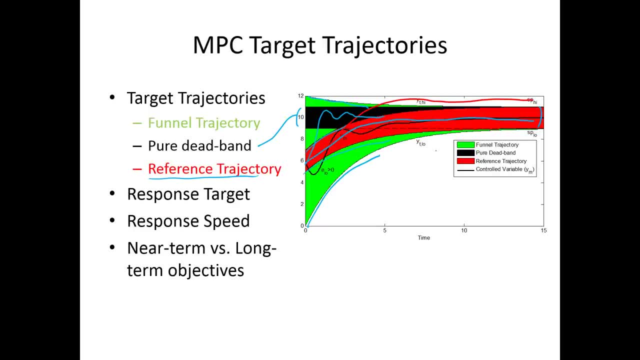 or the controller's doing a good job. Okay, so with this, by adjusting these different trajectories, you can control. you know the final target range. you know, make that as narrow or as wide as necessary. Okay, Okay, Okay. 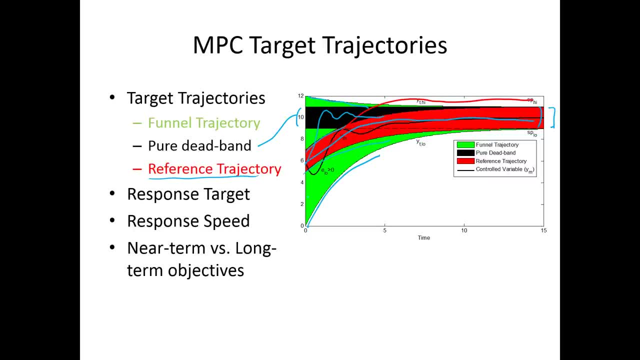 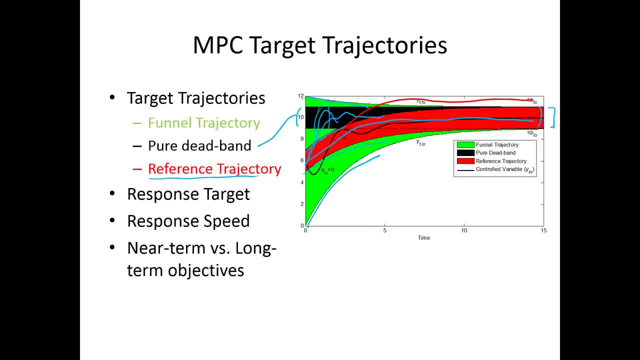 And then also you can prioritize the near term versus long term objectives. Okay, So that one the funnel has you know it says don't be concerned about any of the near term dynamics. Just get me to my final steady state versus the reference trajectory in the red that says we'll try to follow this trajectory coming up. 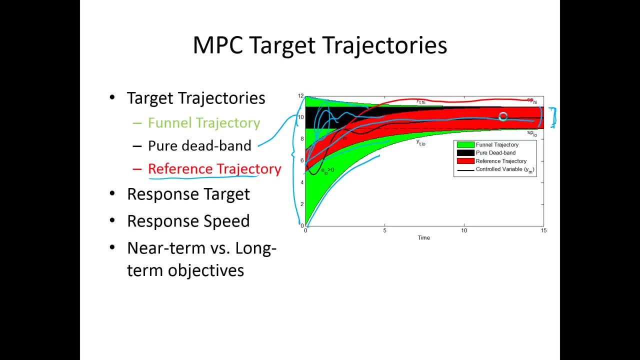 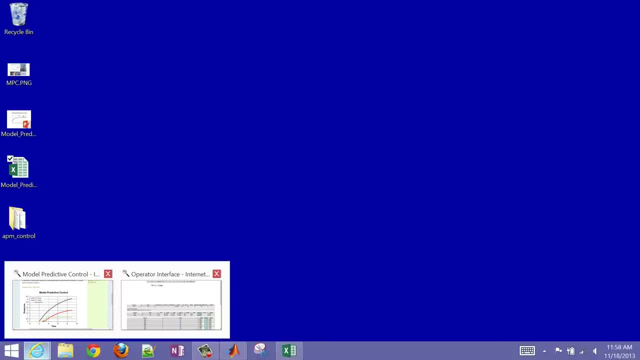 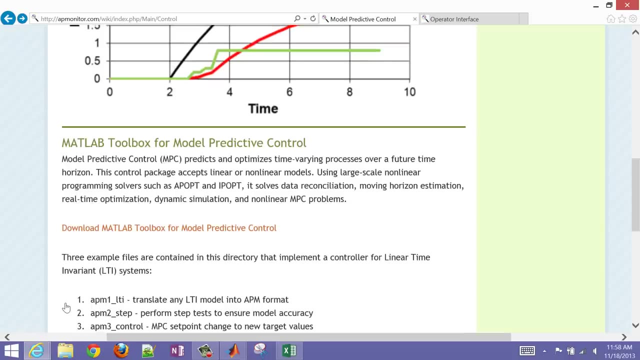 Okay, up to the new setpoint. okay, so let me go ahead and just open up a an example MATLAB script. I'll just come back to the website and just just show that you can. you can download this. this is a MATLAB toolbox for model predictive control and. 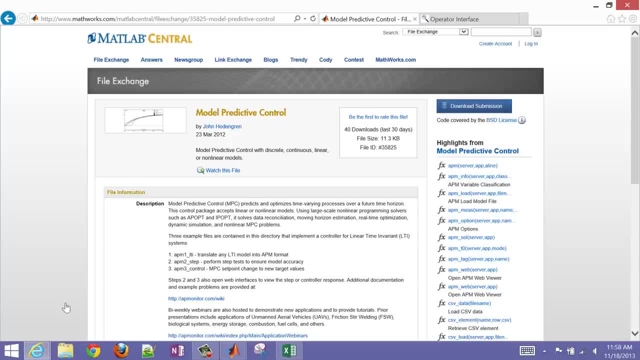 if you visit this, it'll take you to the MATLAB central. now, this is a file exchange site, okay, so you can just go ahead and download, download the the files here and then be able to run this tutorial exercise. what I'm going to do is let me just go back. okay, so there are three files. they're contained in this. 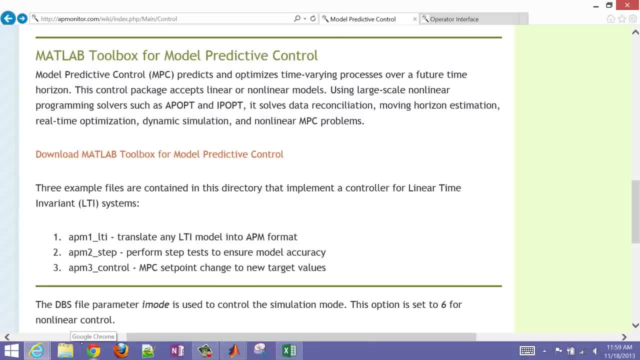 trajectory that you want to run APM one LTI and that'll be able to translate a model into what is called the, the APM format. okay, so this is a text file representation of your model and then we'll show some control calculations. okay, so this is a text file representation of your model and then we'll show some control calculations. 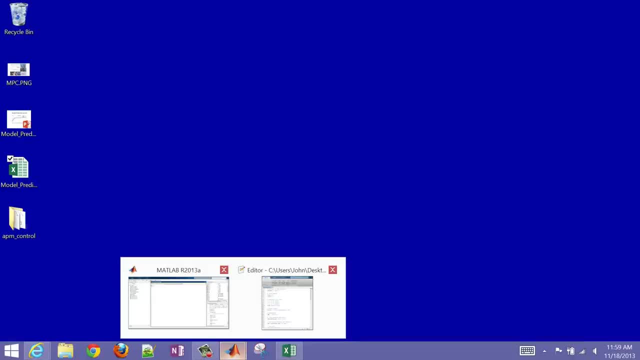 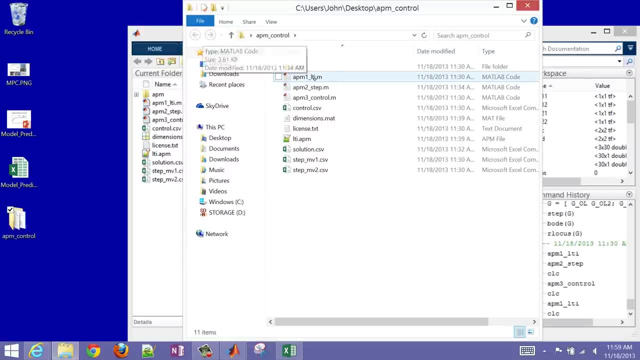 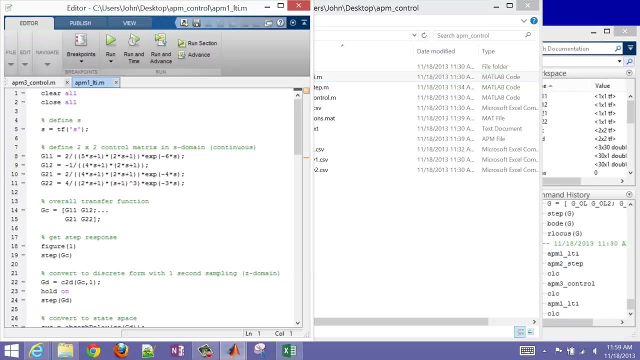 as well. okay, so let me come back here to MATLAB. okay, so I've, I've extracted. I've extracted these files in this folder xh's the first one that we want to work with me. go ahead and open that, open up this file. so what I've done is, you know. 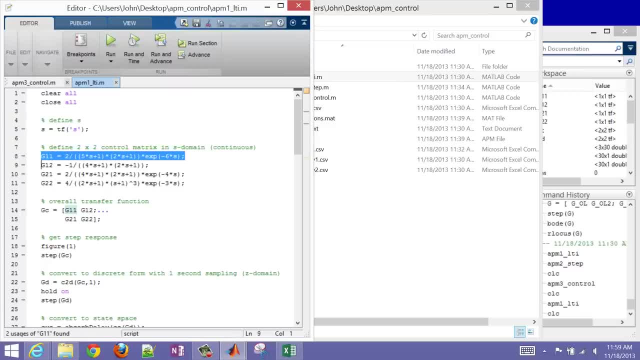 this is just a two input, two output system. okay, so I have just a little plus-a manide to find these transfer functions And then I basically put these into an overall transfer function, a MIMO transfer function- two inputs, two outputs- And then I'm going to plot the step response, convert it to a discrete form. 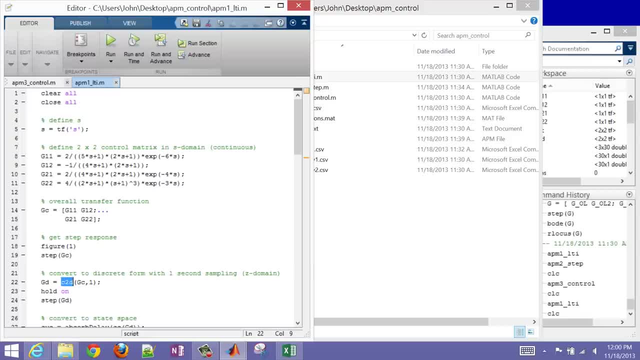 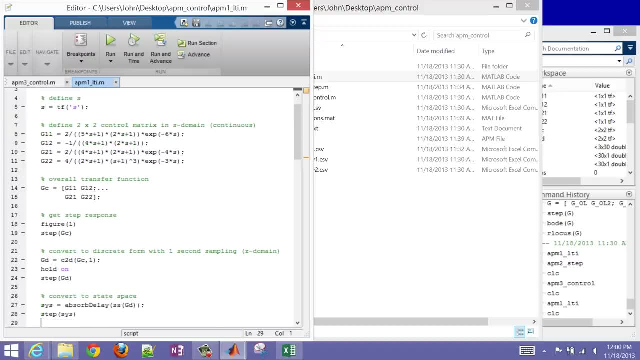 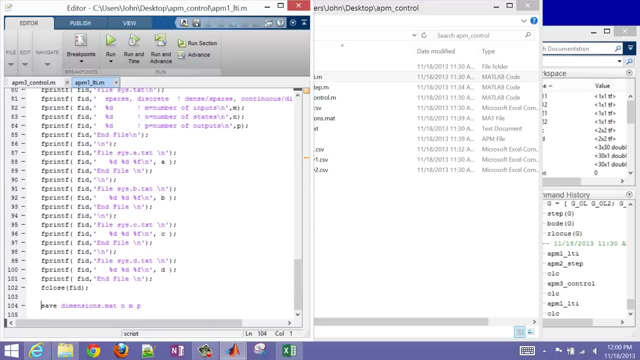 Okay, so that's the C2D function here, with one second sampling, And then also plot that step response, And then I'm going to convert it into the AP Monitor modeling language format. Okay, and then be done with this script. Okay, so let me go ahead and just run this, hitting F5 or the Run button. 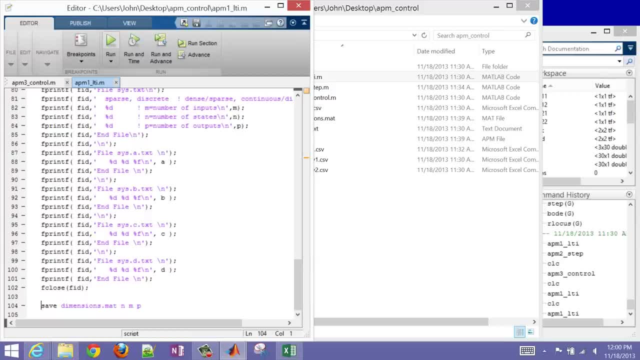 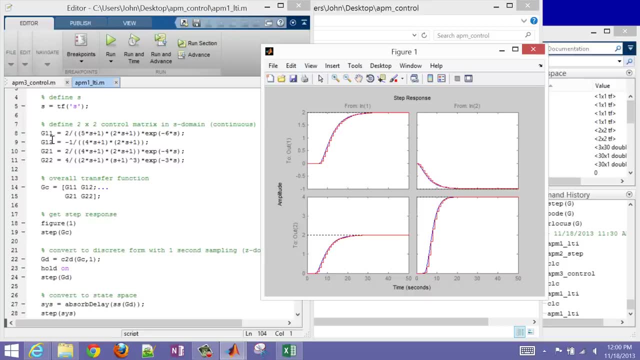 And then we'll see what this model comes up with. Okay, and if I come back up here to the top again, these are the models that I had. So G11 was the relationship between my first input and my first output. Okay, so that had a delay of about six seconds. 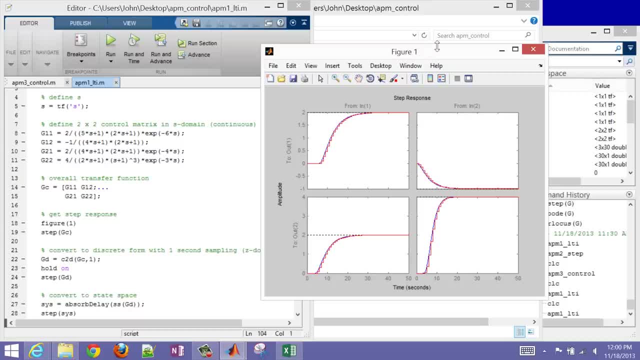 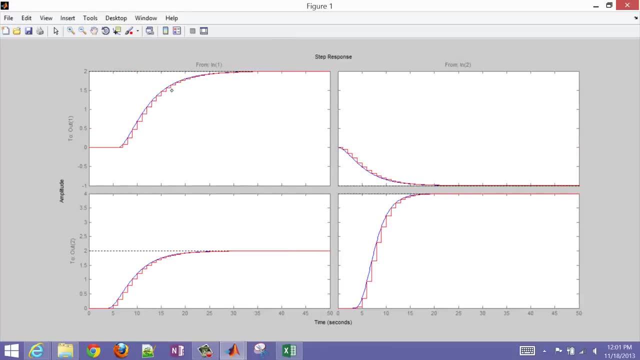 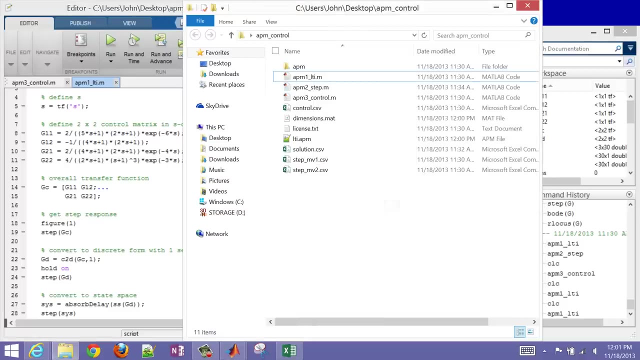 And then you can see the response: The red line here on this plot, that is the discrete model, versus the blue line, that's the continuous model form. Okay, so there I have my model and it's been translated into – actually, let me open up the wrong file there. 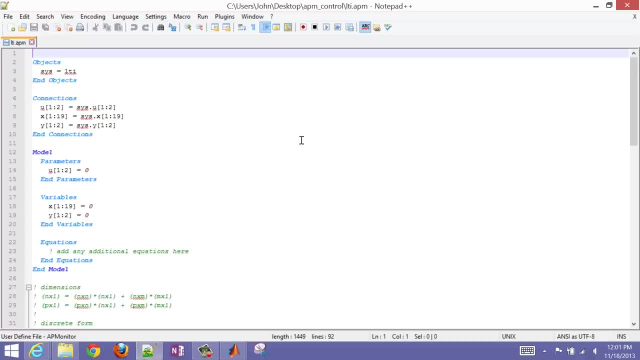 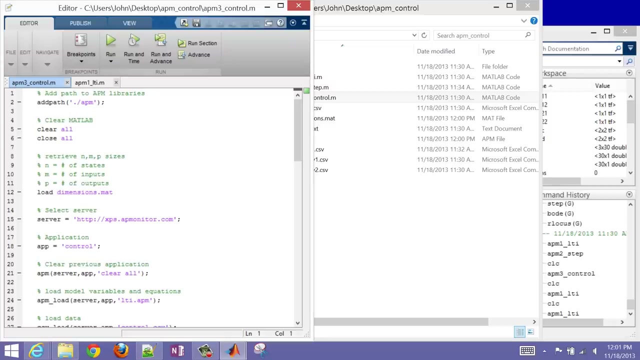 Okay. so if I come back here to LTIapm, this is the model that it translated. This is the model that it translated into AP Monitor modeling language format. Okay, now I'm going to run this, the control calculation. Okay, and this is going to use that same model. 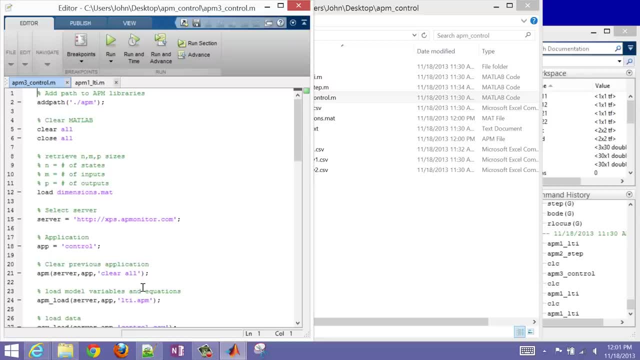 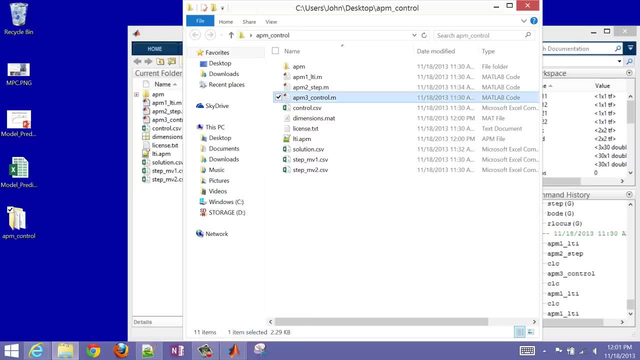 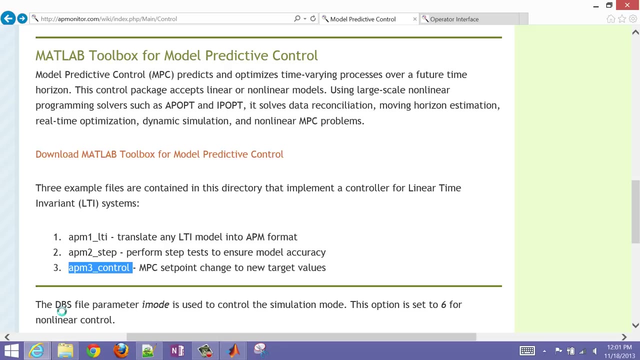 It'll go ahead and load it in right down here in the APM file and then solve this for model predictive control. So this is two inputs. two outputs run through MATLAB, And let me go ahead and just open up The results here on the operator interface. 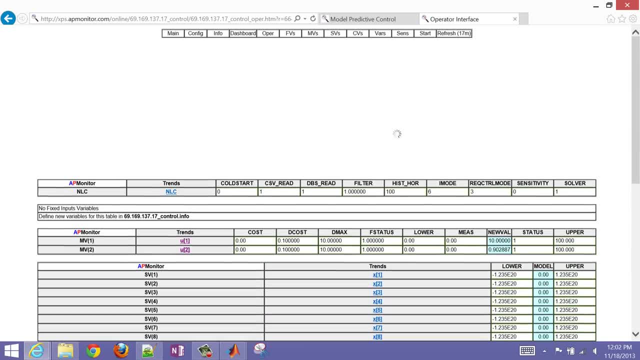 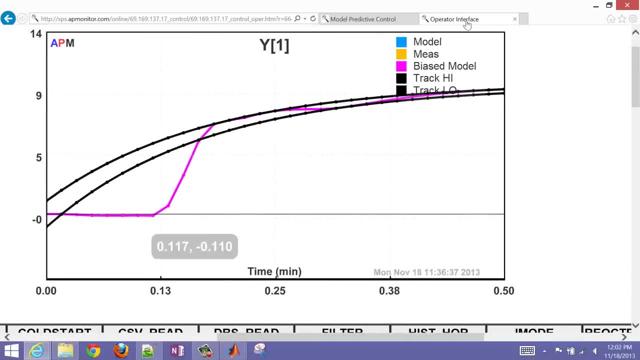 Okay, so this pops up at the end And then I can see that I'm trying to control this controlled variable to this target. Now there's a little bit of a delay here. Okay, now this is listed in minutes, but you can see that it tries to make it up to this reference trajectory right here. 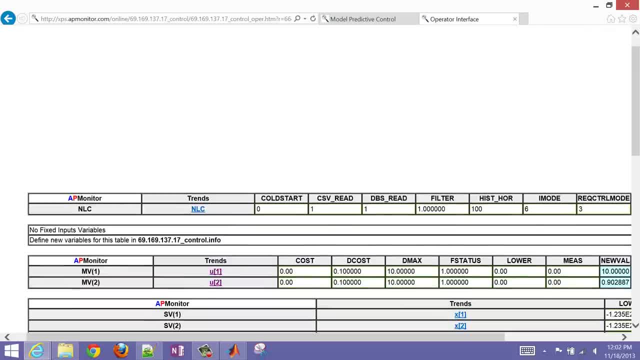 And in order to do that it had to adjust the first input In this way. Okay, so the first input came up down and then steadied out, And then here's the second input as well. Now, this one had just a little bit more complicated scheme.